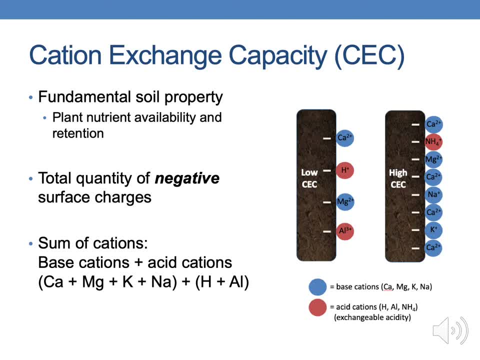 property cation exchange capacity. It's the ability that soil to retain nutrients and supply nutrients to the crops. It's really a measure of charge. It's a negative- the total quantity of negative surface charges on that soil, and it's measured commonly in soil testing labs by summing. 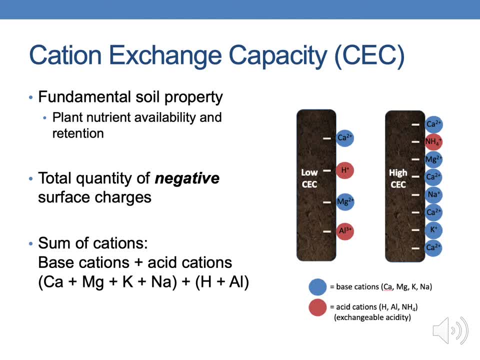 cations. You'll hear that CEC was measured by sum of cations. What that means is these cations, these negatively charged ion, or, sorry, these positively charged ions such as calcium, magnesium, potassium and sodium. These are our base cations. Then we have 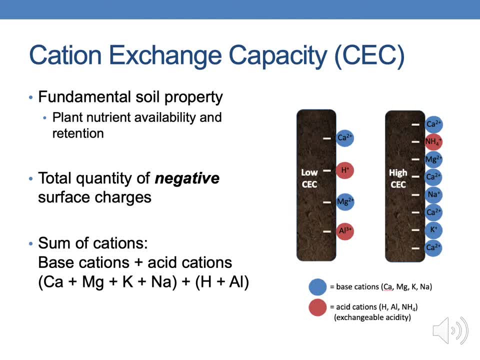 acid cations, including hydrogen, aluminum, ammonium, manganese, iron, etc. So we have both basic and acidic cations and they all have positive charges and they stick to the soil. They adhere to the soil because they have a positive charge. So they stick to the soil because they adhere to the soil. 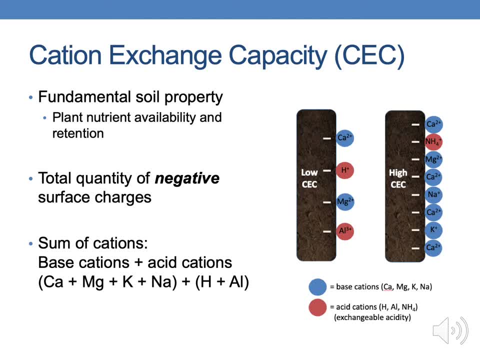 Soils are typically negatively charged, and so that's why CEC is such an important property. The picture over here: on the right we can see a low CEC soil with a few- not very many- negative charges and the associated positively charged cations attracting to them. Then on the very right, we 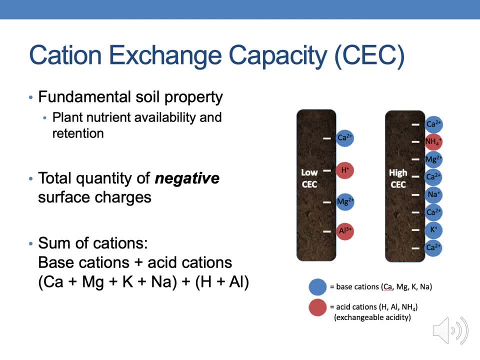 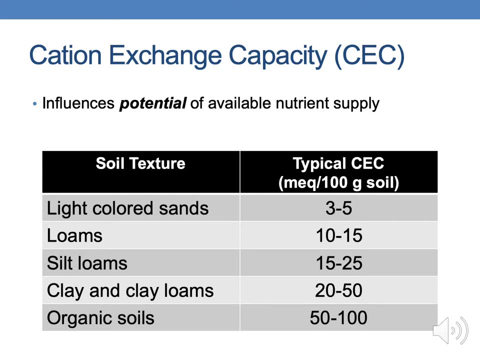 have a high CEC soil with a lot of negative charges and you can see the cations, both positive, both, sorry, both and acid cations attracted to that. So CEC is it's important to notice, it's a potential of nutrient availability and supply, but it's not a particularly a direct measurement because the nutrients could. 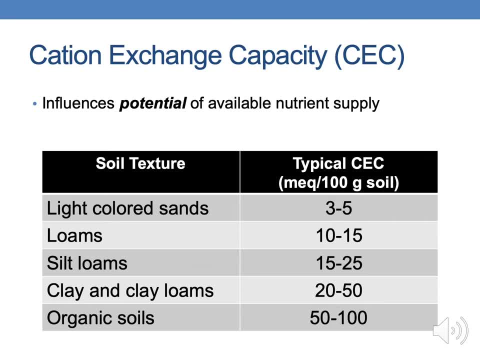 be there, but they might not be right. So, and just to give you some idea, it's driven really strongly by soil type and primarily by clay content. Okay, so here's just a range of CEC values that you might encounter, Three to five with the really sandy soils, Most of the soils that we find in the Midwest. 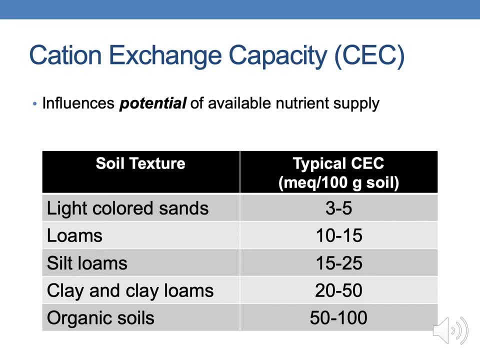 and Ohio would be somewhere between 5, 10 and 25.. So in these loam, silty loams, we get above 25 and they really started getting to heavy clay soils, very heavy clay soils, and even into the organic soils or the muck soils, So that you can see the. the range can be quite quite large. Now let's talk. 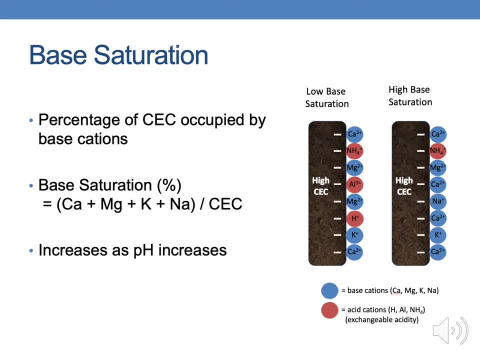 about base saturation. Okay so, base saturation is the percentage of CEC occupied by base cations. Okay so again, we can define this as our calcium, magnesium, potassium and sodium divided by CEC. So it's a percentage of the CEC, the percentage of the CEC that the bases actually represent. This is going to increase as base cations. 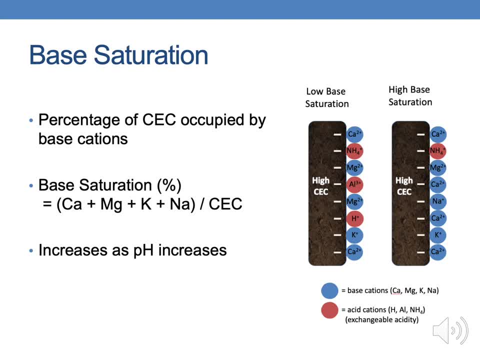 increase and base saturations increase, our pH is, by default, going to increase, Okay, so. Second, we then have CEC S3, where we have a low base saturation and a high base saturation, But we have a situation where we look at this picture again, We look at this picture: we've got a high CEC. 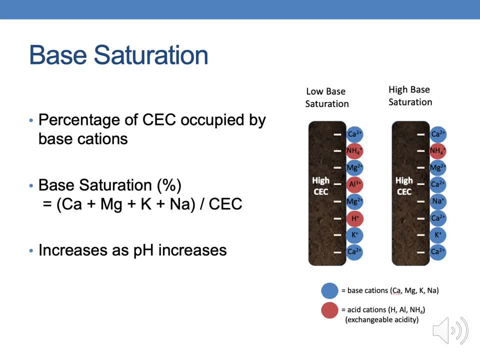 soil with a low base saturation and a high base saturation. So the difference between these two is that the one on the left, the low base saturation, has a more acid cations or exchangeable acidity occupying those exchange sites. The one on the right has lesse, So the pH on the right will have higher base saturation. 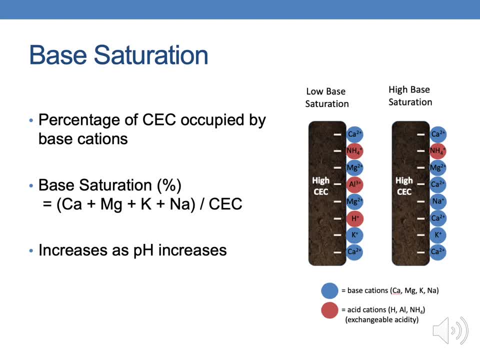 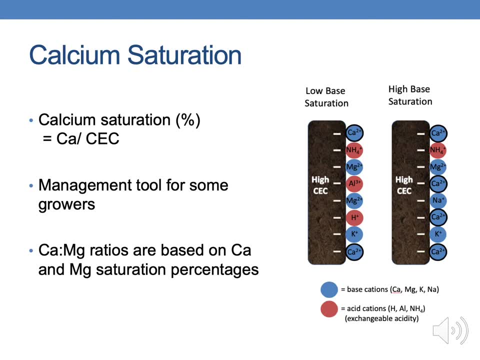 higher pH, Low base saturation saturation, lower pH, and we can also think about calcium or magnesium saturation, etc. etc. so calcium saturation as a percentage is essentially the amount of calcium exchange on the exchange sites, that as a function or as a percentage of the total CEC. so this is a management tool that some growers use. 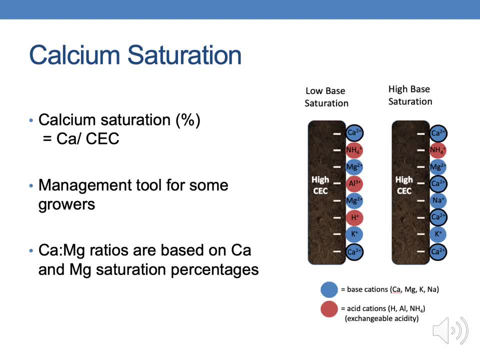 heavily and pay quite a bit of attention to how much of the exchange site is calcium, how much is magnesium, and we can often calculate calcium magnesium ratios. these are all soil test results and this is essentially a ratio of the calcium to magnesium saturation percentage. okay, so again, there's a lot. 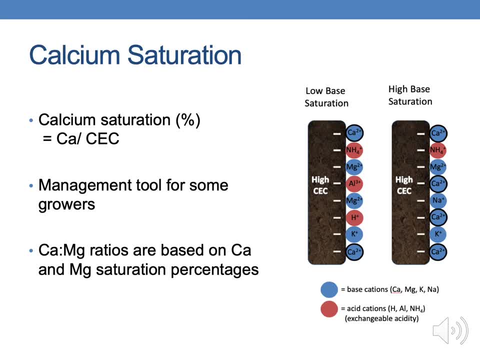 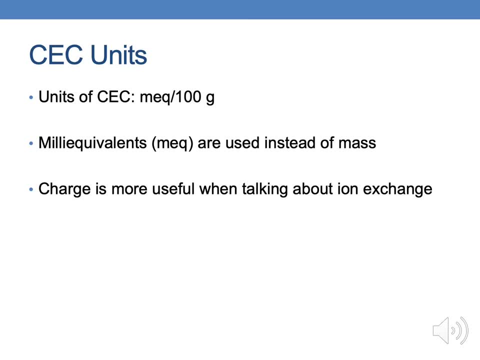 of management applications in terms of how people think about and are using their soil test information. CC units are kind of an interesting beast. Technically, the unit that you'll get on most all-soil tests is a mill equivalent per 100 gram of soil. 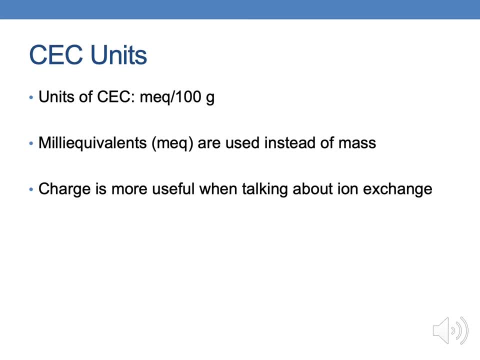 So what does that actually mean? Well, mill equivalents are a measurement of charge and they're used instead of mass. So if you look at, say, percent organic matter, that's a mass of organic matter per mass of soil. Here, with CEC, we're talking about charge, charge per mass of soil or charge per weight of soil. we could say: 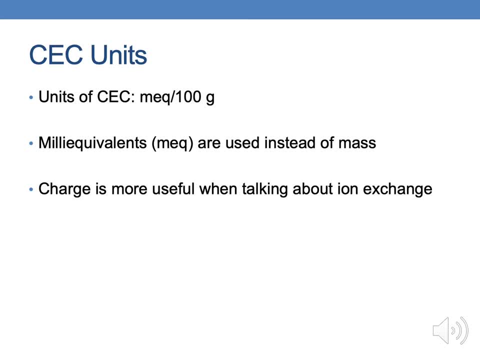 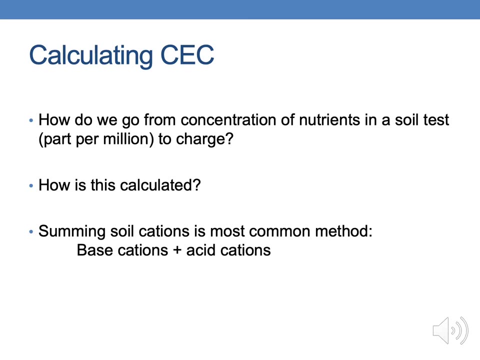 So charge is more useful when talking about ion exchange than, say, a mass percentage. So that's why we use this kind of funky unit of mill. equivalents per 100 grams. So again, it's a charge per weight of soil. So the question is, how do we go from a concentration of nutrients? 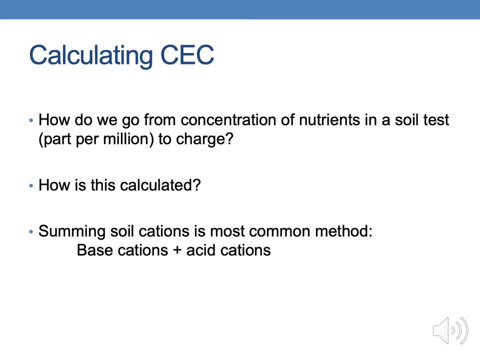 When we actually submit a soil sample and have a soil test, they actually extract and quantify the concentration of calcium in that say, malic-3 or ammonium acetate extraction, The concentration of magnesium, et cetera, et cetera. 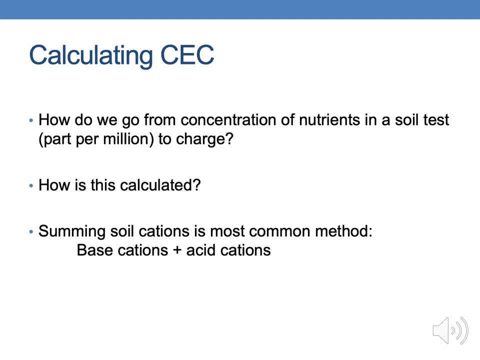 And that somehow gets magically converted to a CEC number. Well, we're going to do a little bit of a deep dive right now to talk about how that's actually done. So again, we're thinking of CEC as a summation of cations, both base and acidic cations, and that's what we're going to get into. 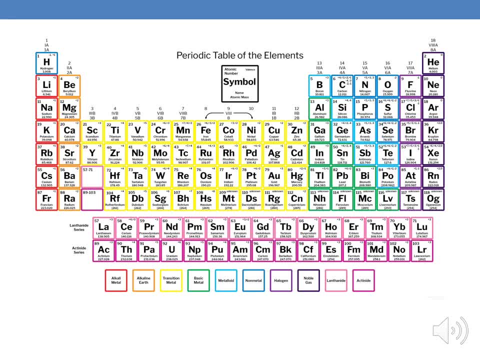 So the periodic table, thinking back again, you know maybe high school or college chemistry, and we've got a lot of different things. We've got a lot of different things. We've got this periodic table. Here are our base cations of calcium, magnesium, sodium and potassium. 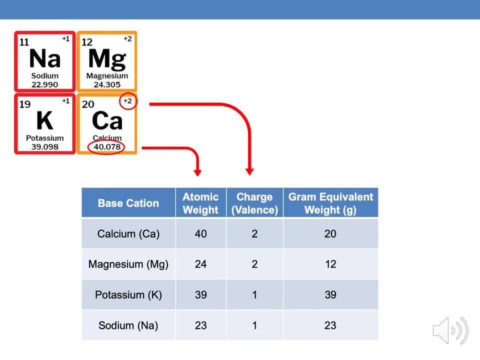 These, at the atomic level, have weights and charges. So calcium, for example, says there's approximately 40 grams per mole of calcium. That's the atomic weight And it's got a charge or a valence of plus 2.. 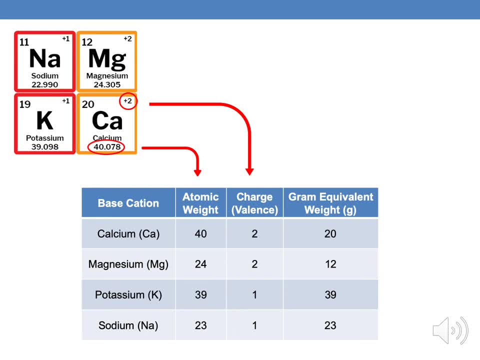 So we can take the atomic weight, divide that by the charge and we get what's called a gram equivalent weight. So one of the things that we need to do to kind of make this make sense and make these numbers line up is that we first have to convert these gram equivalents to mill equivalents. 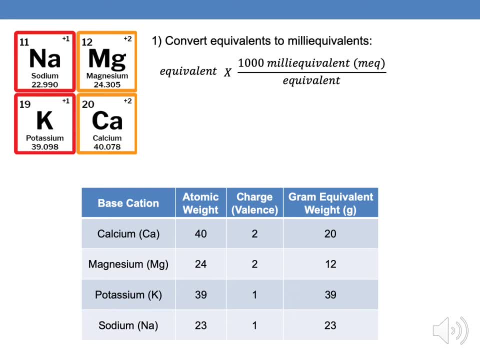 And we do that by taking 1,000 mill equivalents per equivalent and we get again this 1,000 mill equivalents. The second step then is to set mill equivalents for 100 grams of soil. Again, our unit is mill equivalents per 100 grams of soil. 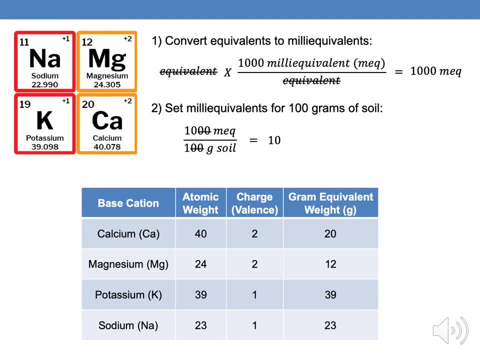 So we do this, Divide by 100, and we have zeros, cancel, and then we get this equals 10.. So this essentially becomes a multiplier that we use. So we take our gram equivalent weight and we want to convert it from a gram equivalent to a mill equivalent per 100 grams of soil. 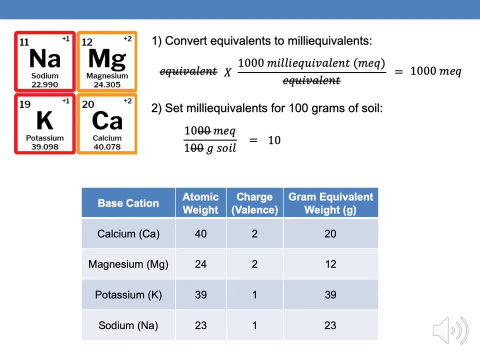 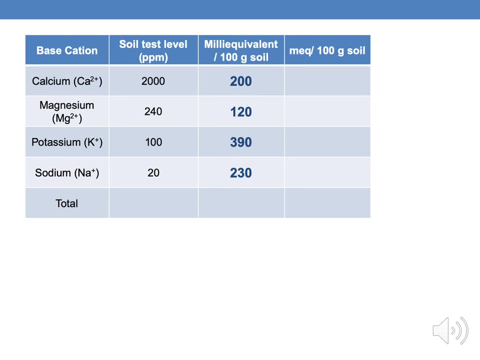 We multiply these values in this rightmost column by 10, and then we get essentially a conversion factor of sorts mill equivalent per 100 grams of soil. So here we are Now. this is really, for the most part, where you can start for a soil test. 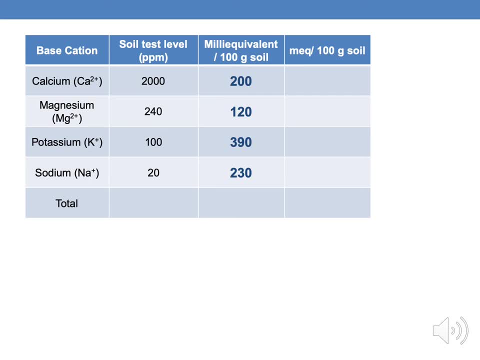 So we get a soil test value. Say it's a malic-3 extraction reported in part per million. We've got 2,000 part per million. calcium, 240, magnesium, et cetera, et cetera. Again, here's our conversion factor. 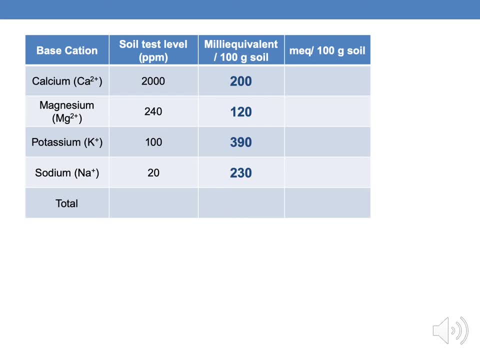 What we do is we divide this soil test level in ppm by our mill equivalent per 100 grams of soil. We're taking it from a concentration in this step, a concentration to a charge. So now we're at. for calcium, we're at 10 mill equivalents per 100 grams of soil. 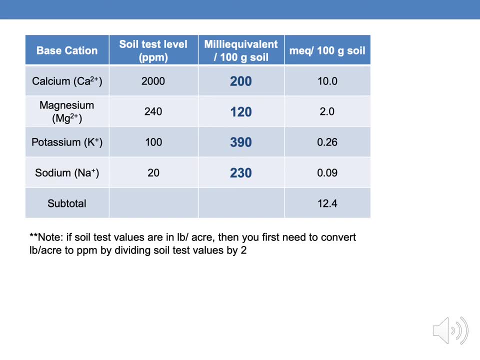 It's important to note that if your soil test levels are in pounds per acre and not ppm, you first need to convert from pound per acre into ppm, most commonly by dividing by 2.. So if it was 4,000 pounds of calcium per acre, malic-3 extraction. 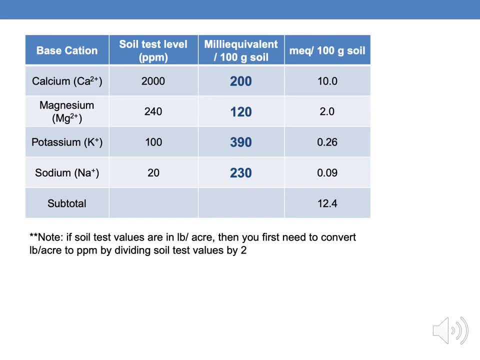 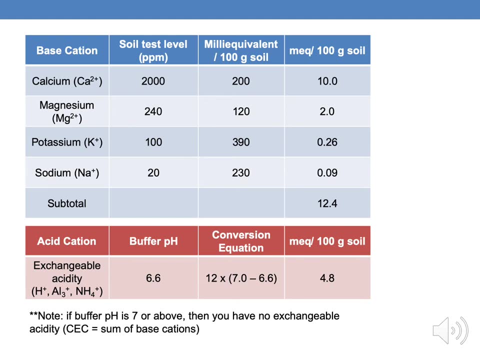 then we're going to divide. We're going to divide that by 2 and get it back to 2,000, okay. So then there's this acid piece. okay, So this exchangeable acidity is also important, because we know it's not just these base canines. 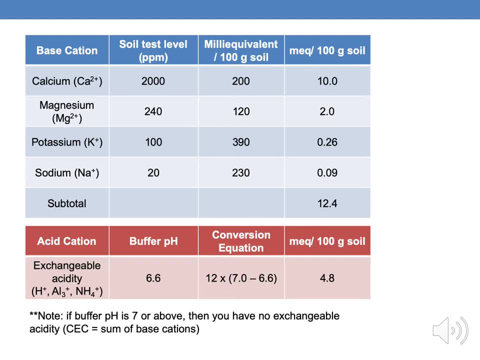 There's also acidity very commonly in our soil. So we do this- and this is a bit of a magic box here, but there's an empirically derived relationship- that has been used for Ohio soils And we do this by taking the buffer pH. 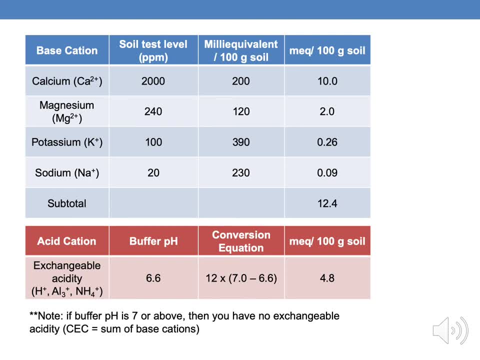 and we do this by taking the buffer pH in our soil test. That again is our soil that's had a little bit of liming solution added. and then we measure pH. We take that, we divide that buffer pH by 7, and we multiply this by 12,. okay, 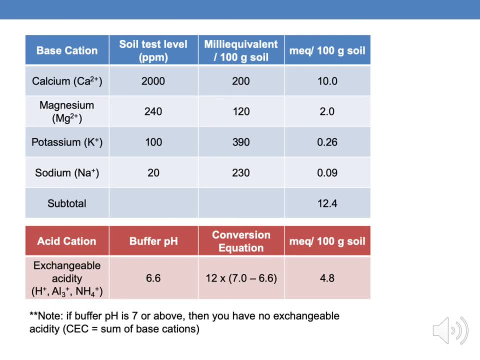 And that gives us this value of 4.8 mill equivalents per 100 gram. So it's important to note that if our buffer pH is at 7 or above, some soil test reports will just say 0 for buffer pH. If it's 7 or above, this becomes 0,. 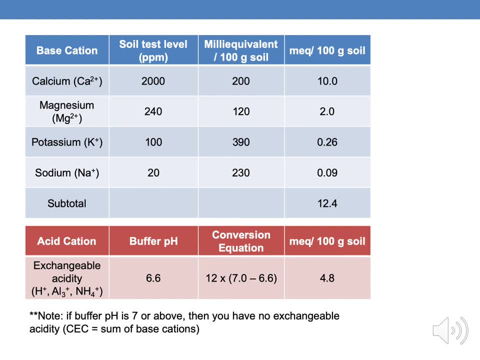 and then we essentially don't have to worry about the exchangeable acidity. So if we do have exchangeable acidity, which this soil test indicates we do, then what we do is we're going to add our base canines here, which is the 12.4, and our exchangeable acidity at 4.8.. 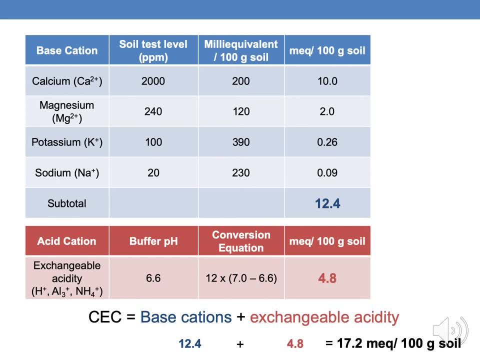 And our value, our final value for CEC is 17.2 mill equivalents per 100 grams. So that's that. So that's really the step, And again we can kind of eliminate those first few slides when we're talking about periodic table. 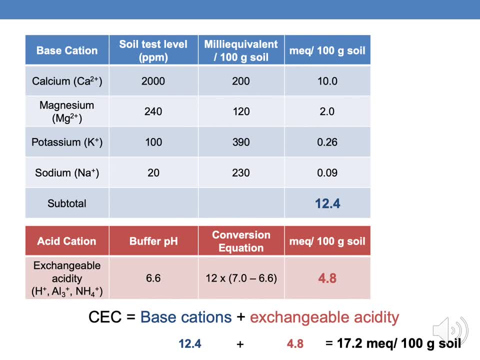 just using this conversion piece, taking our soil test level, dividing it by our mill equivalent per 100 gram conversion, and you can get the essentially charge per unit at that point and add those up and you get the CEC. Okay. 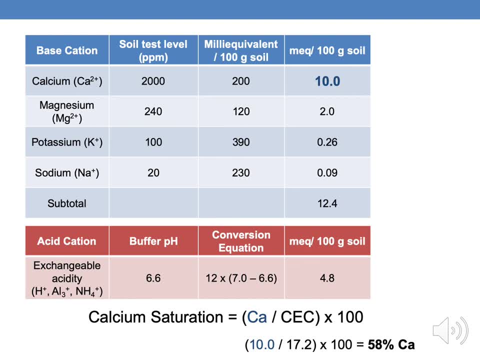 We can also talk about calcium saturation, again by taking calcium, the mill equivalent of calcium divided by the CEC, And so in this example, 58% of our exchange sites would be calcium. We can do the same thing with magnesium. 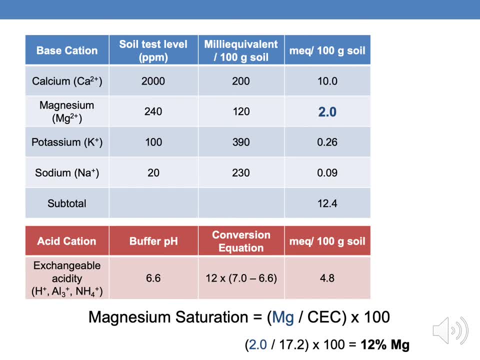 So instead of 10, we're using 2, 2 mill equivalents of magnesium, and so that would be essentially 12% magnesium. So you know, these are kind of the basic pieces of running through this And so hopefully that gives you a little bit better. 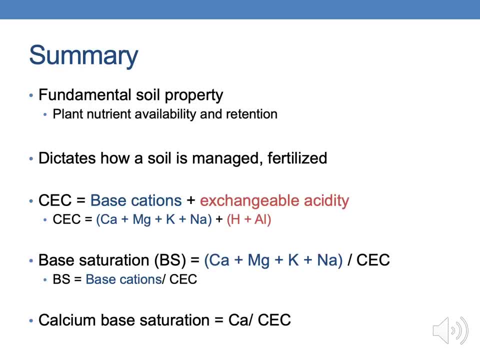 a better understanding of what we're dealing with And just to kind of summarize, I'll say that CEC is a fundamental soil property. It's very important for plant nutrient availability. It really dictates how a soil is managed, fertilized. It's one of the first things that most you know: crop consultants, farmers.